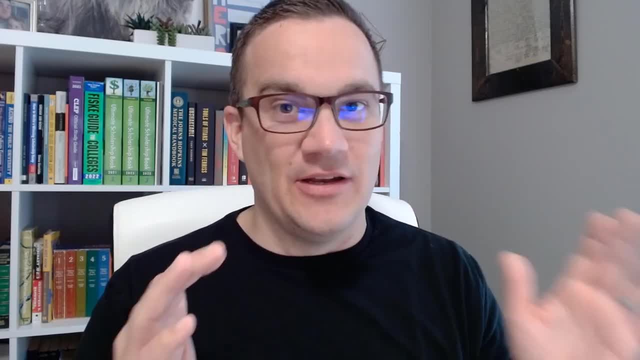 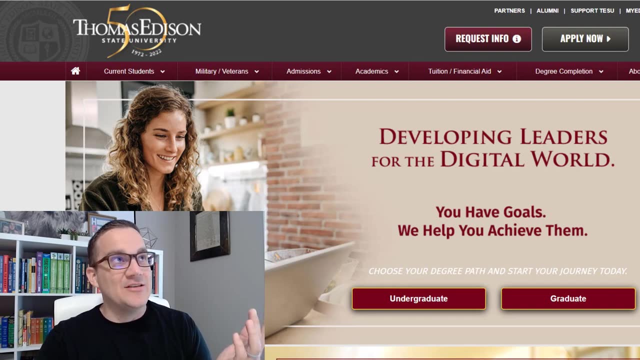 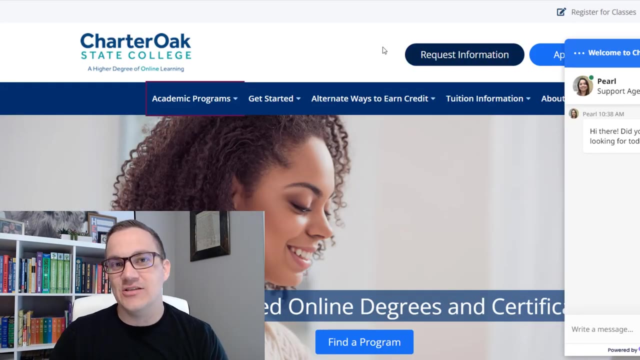 is crazy fast. Let's jump over here. I'll walk you through everything. There are two different strategies you can take First strategy. you can choose a school like Thomas Edison State University, Excelsior University, Charter Oak State College. These are schools, and there are a number of others. 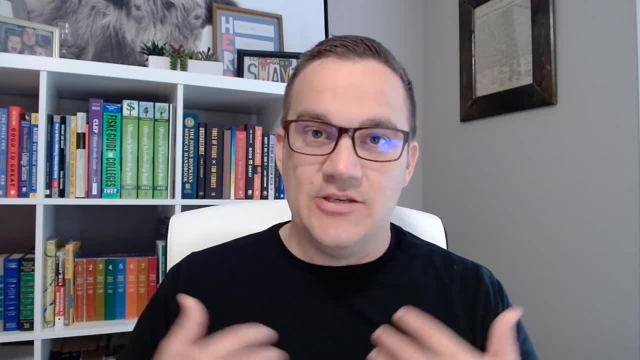 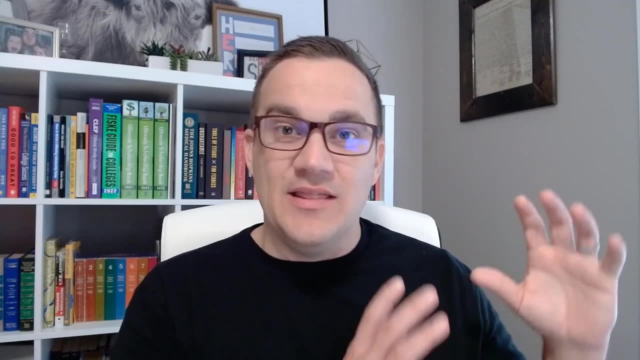 that are really flexible with transfer credits So you can go earn like a bunch of credit through things like CLEP exams, sophiaorg studycom. This is one method to graduate faster, but in my opinion it's a lot faster. So I'm going to walk you through everything. There are two. different strategies you can take. First, you can choose a school like Thomas Edison State University, Charter Oak State College. These are schools- and there are a number of others- that are really flexible with transfer credits So you can go earn like a bunch of credit through. 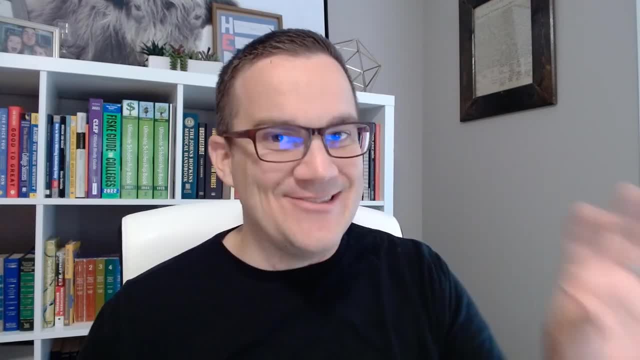 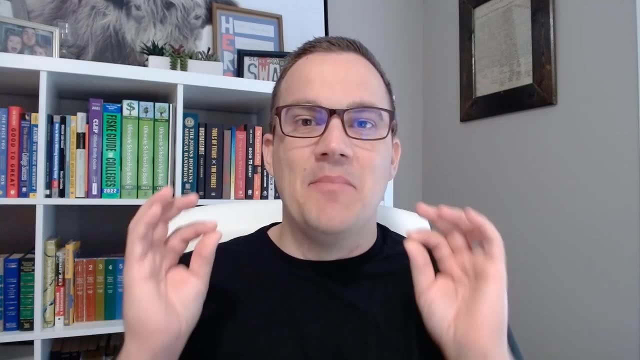 things like CLEP exams, sophiaorg, studycom. This is one method to graduate faster, but in my opinion there are faster ways to earn college degrees. This is not my favorite approach to earning college degrees. It's the most well-known approach to accelerate, but in my opinion 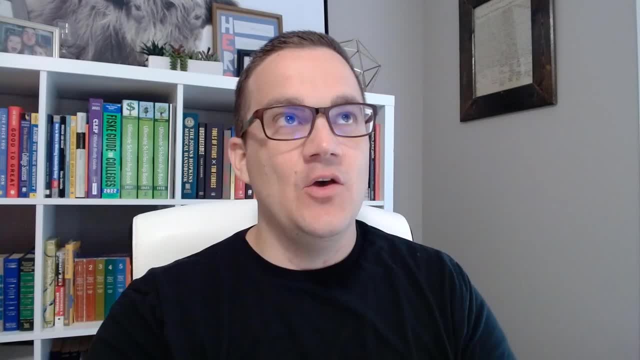 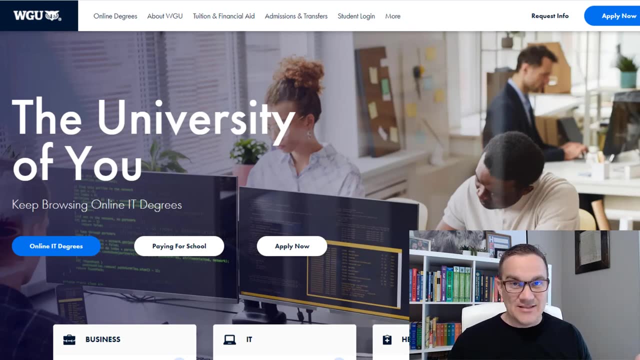 it's not the best. Now, approach number two would be to find schools that are 100% competency-based and 100% self-paced, with no limit on how fast you can graduate- Schools like Western Governors University, University of Maine at Purdue and other schools like that, So you can go. 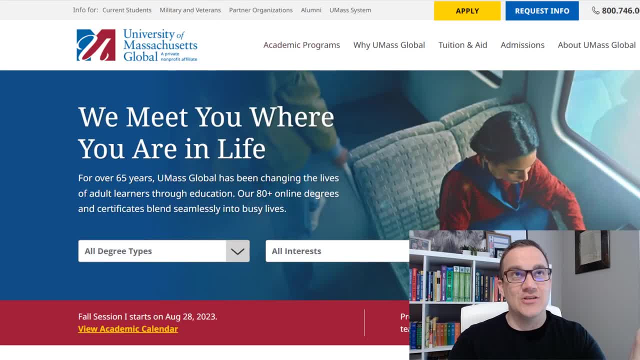 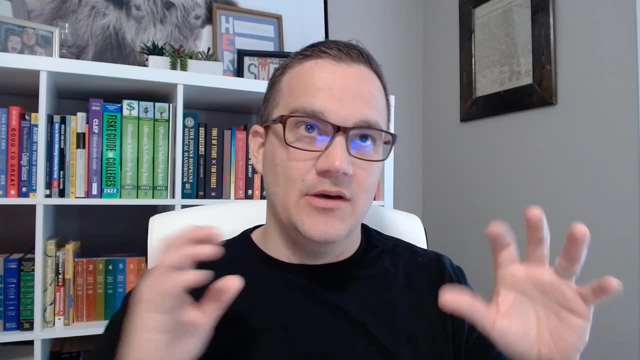 university of Maine, at Presque Isle University of Massachusetts, Global has some programs like this and there are others, but here's the difference between the two approaches. Approach A that I talked about: you're earning your credits through third parties and then transferring them. 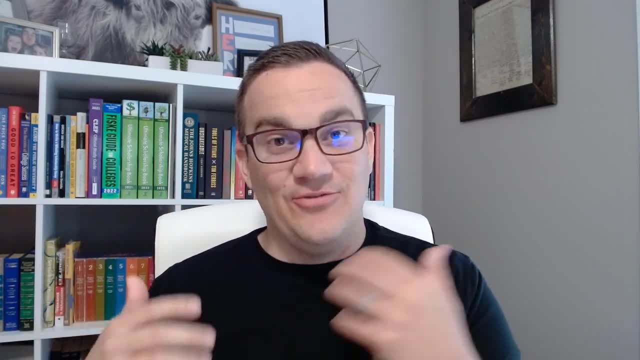 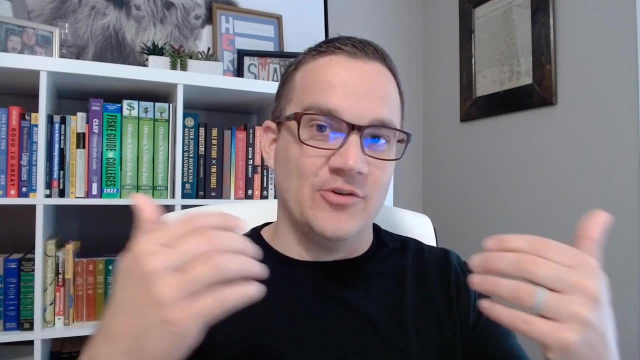 over to the schools. Approach number two is you're finding schools that allow you to accelerate inside their programs and you're doing all of your degree hacking through the school. Well, in my opinion, it's a lot faster. So I'm going to walk you through all of these. 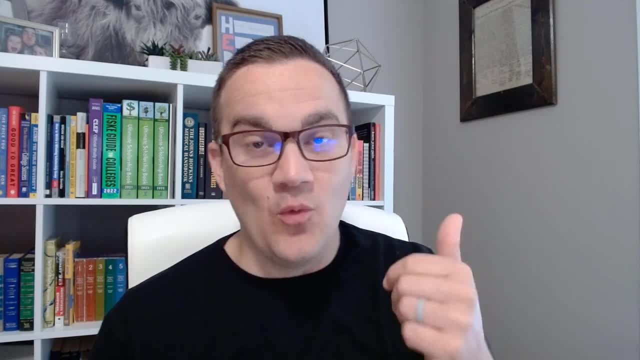 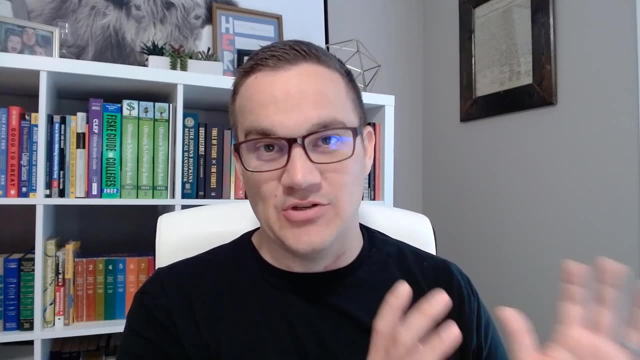 in my opinion, I like this approach better for a couple of reasons. Number one: you can graduate faster, okay, And the reason being most schools that are really flexible with transfer credits, they have rules saying, hey, we'll accept up to three years worth of. 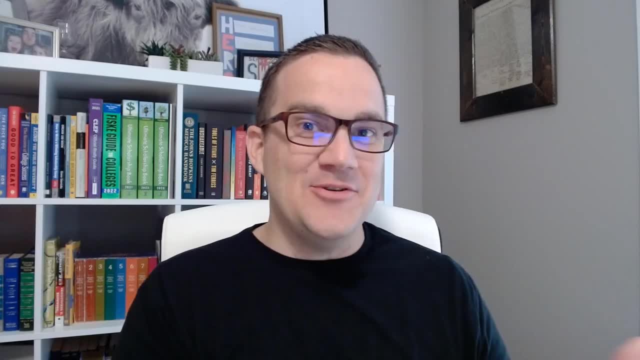 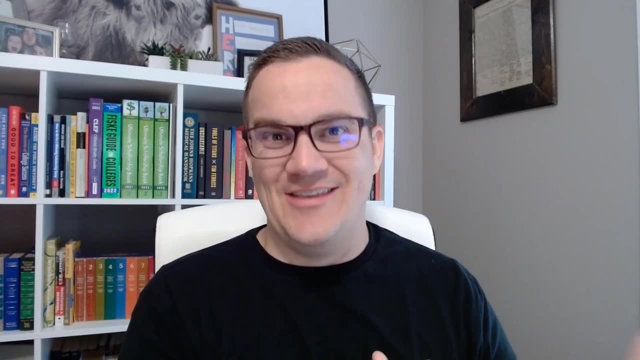 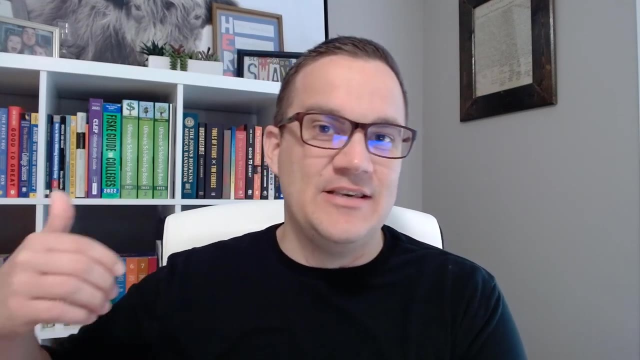 transfer credits, but then you need to come do a year through our school as a more traditional student, So you're going to earn these transfer credits really quickly, and then you got to go to a whole nother year through the school. Well, these competency-based schools, the ones that have zero limit on how fast you can go- 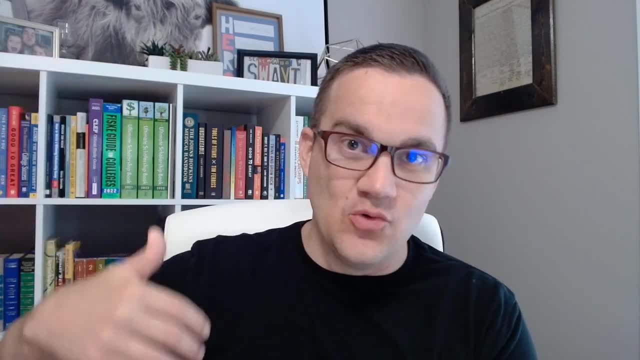 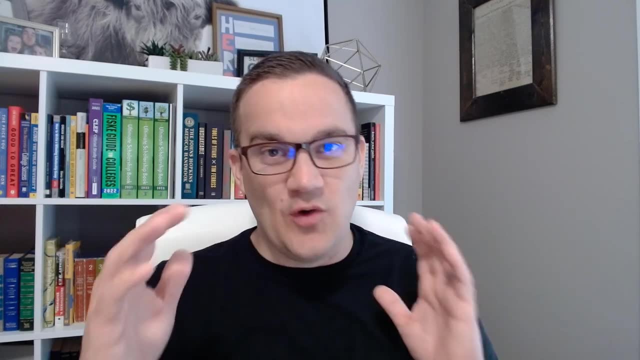 through classes. you can just go hack everything through the school and you can get it done significantly faster. Like I said, I've seen as fast as three months. six months to 12 months is pretty normal for people that work with me, But that's the thing is, if you're doing it. 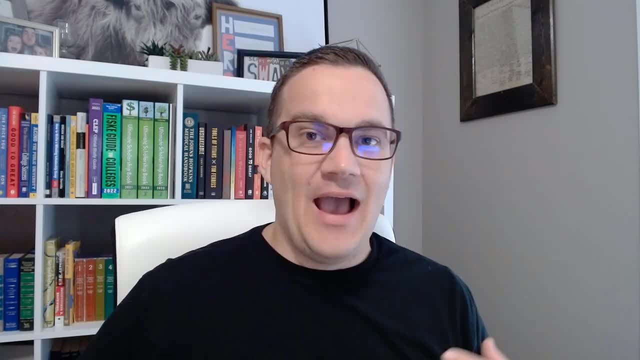 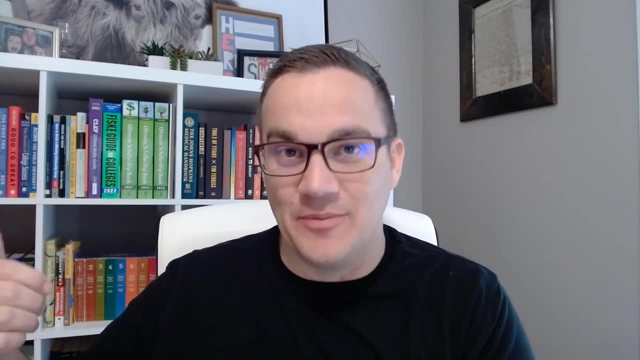 through the school. some of these schools don't have any limits. Having said that, there's two strategies. I think my personal opinion and from my experience- I've helped a lot of people do this. From my experience, hacking through competency-based education programs tends to be. 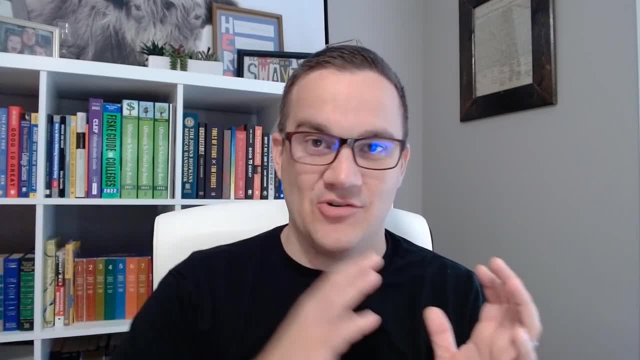 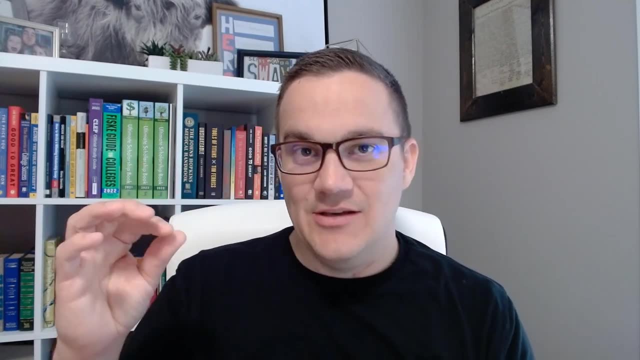 faster and cheaper, because the faster you graduate, the less you pay in tuition, because most of these schools charge you per semester instead of per credit. So if you have that flat rate tuition per semester you can go faster. So that's my faster method. as far as choosing which, 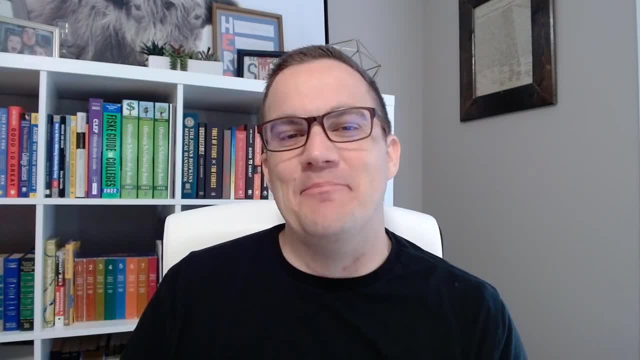 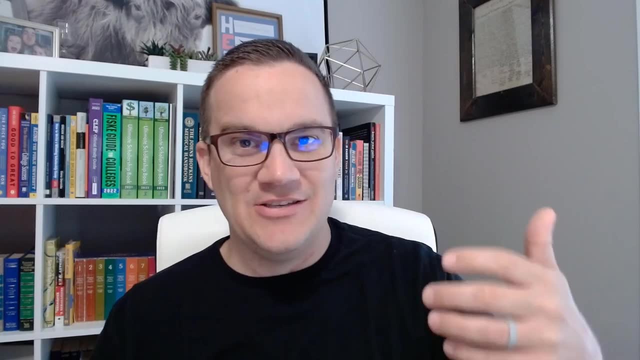 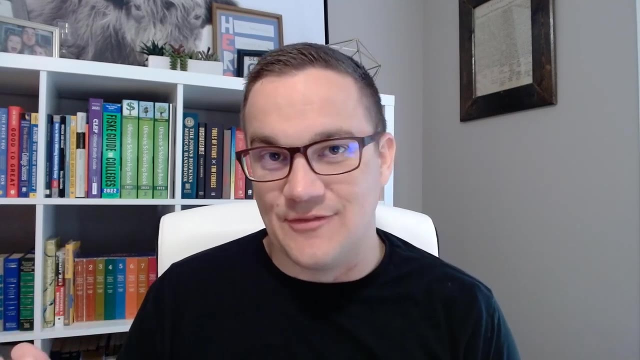 strategy. but what majors? okay, There's so many different majors you can choose to accelerate. I mean you can do business degrees and tech degrees and teaching degrees. You can even do degrees related to the health field. You can do, like, seriously, tons and tons of different majors. 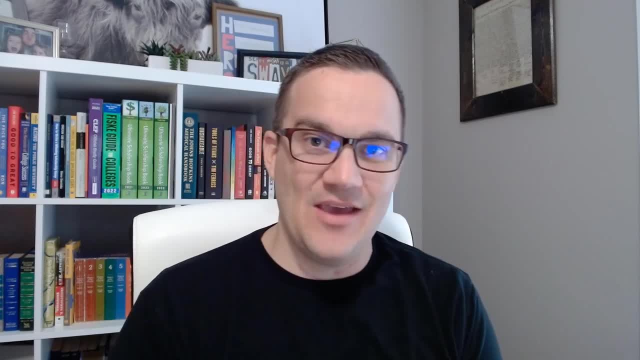 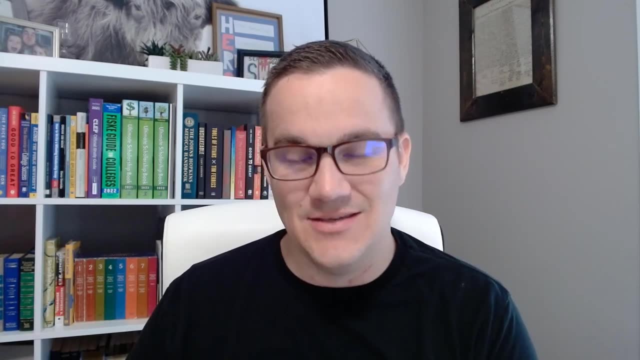 you can accelerate Now. some majors are math heavy, Some majors are science heavy. Some majors are English heavy, where you're writing lots of essays. Some majors are math heavy, where you're writing lots of essays. Some majors are math heavy, where you're writing lots of essays. Some majors are 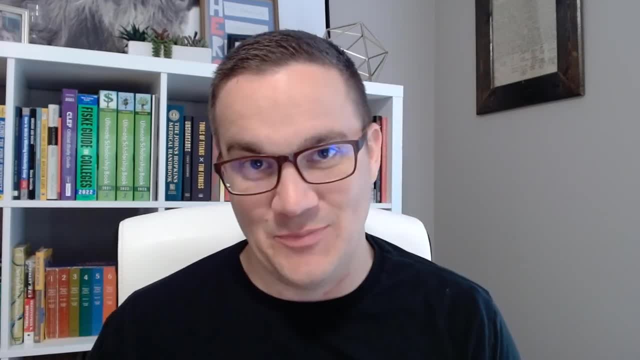 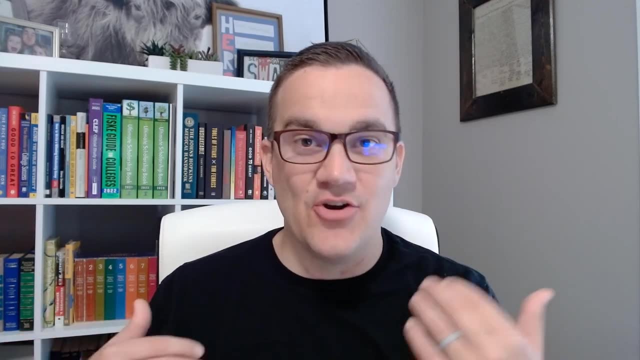 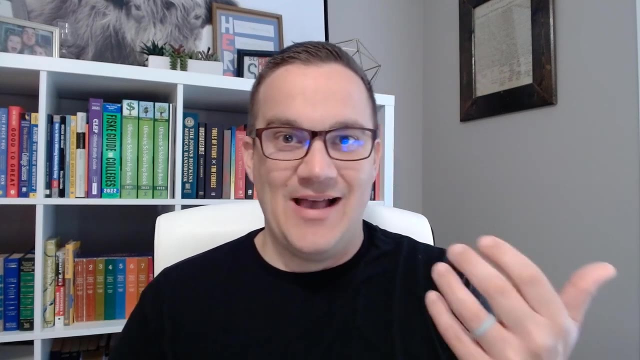 faster than others, and here's my opinion, just from my experience. I think business majors are way faster than other majors. Let's say you're going to do a tech degree. okay, Well, tech degrees: you have to learn the tech, You have to have classes related to coding, You have to have 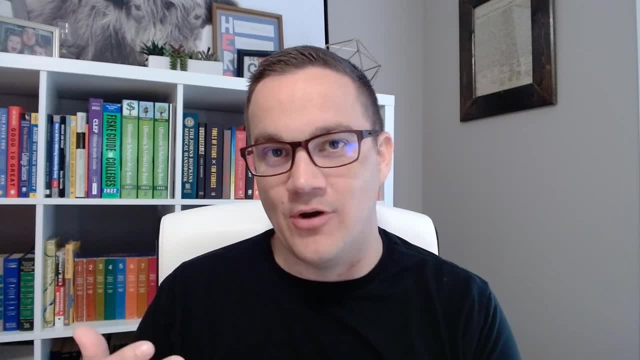 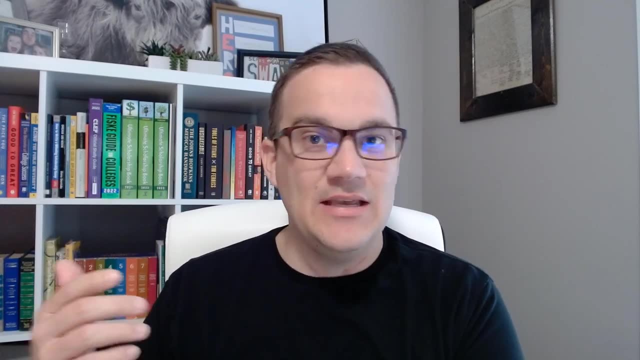 all these different classes that for some students are foreign. Now, for some students, if you're just a tech whiz, tech might be the fastest lane. okay, Then you have other majors. Let's say you want to get a teaching degree. You're going to have to do more math, more science. 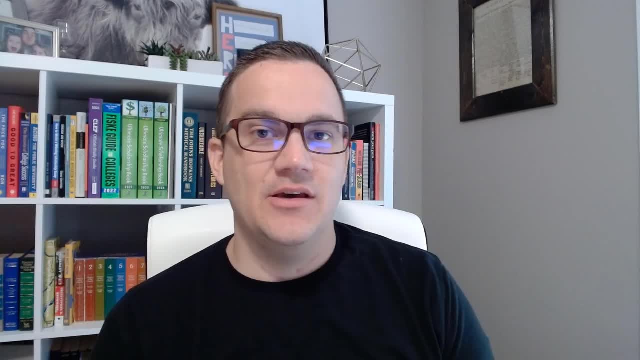 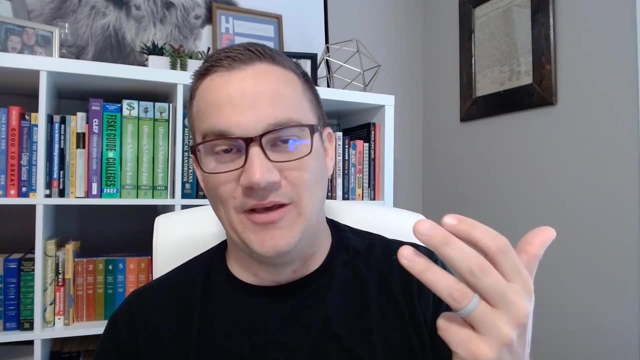 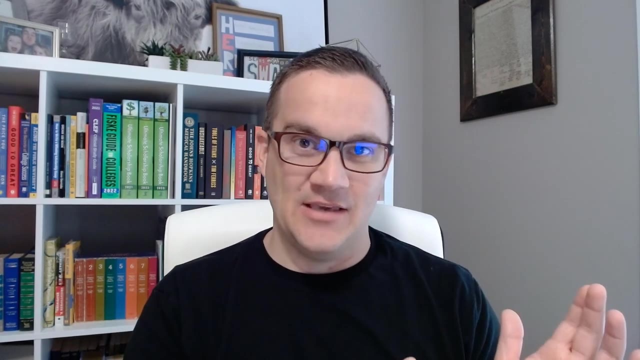 more English than a business degree. Business degrees, they're basically your bare minimum math, bare minimum science, bare minimum English, bare minimum history. and then business classes are pretty easy, and let me tell you why. Business is one of those things that, if we live life normally, 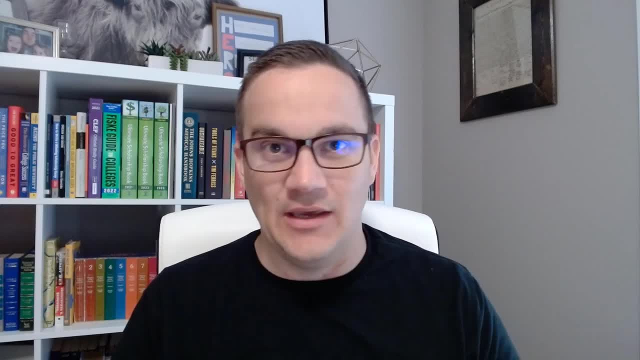 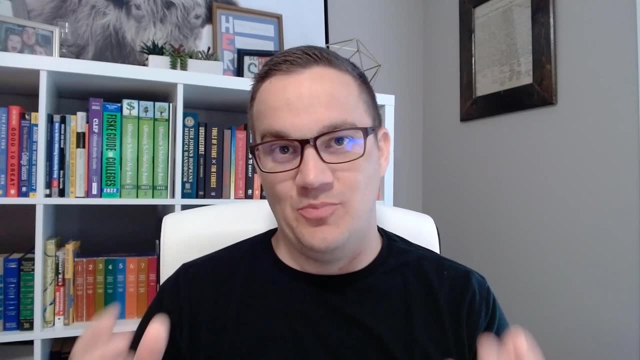 we are around businesses all the time. We're walking in and out of stores, We're seeing advertisements all over the place, We're purchasing things, We interact with business all the time. so when you go get a business degree, oftentimes what you're learning- 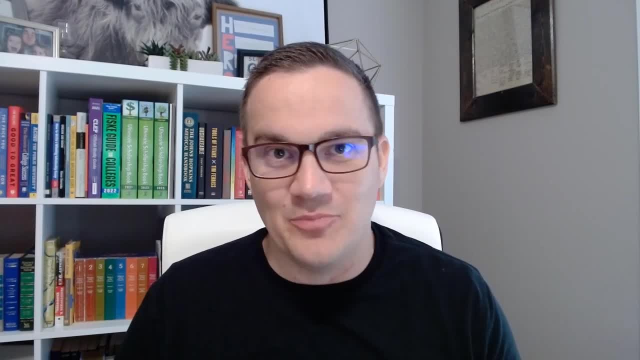 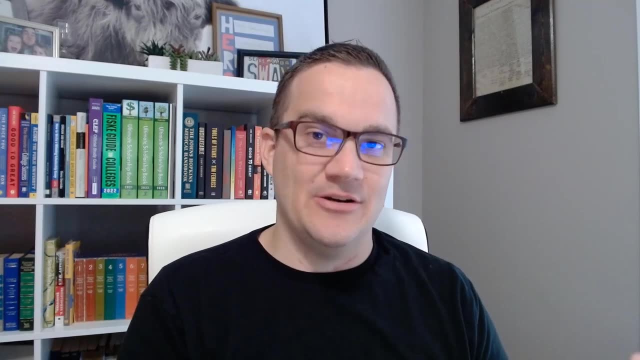 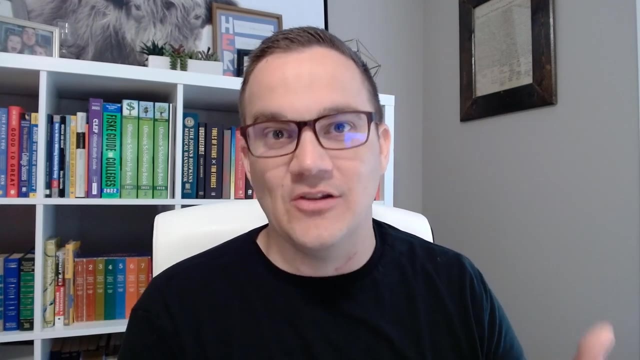 is kind of second nature, because you've been around business your whole life and when you go and try to test out of your classes and go through the material faster, a lot of times it almost seems like common sense and you're not doing as much learning, You don't have to learn as much. 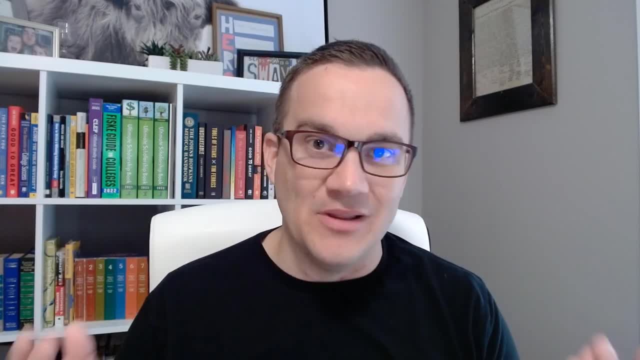 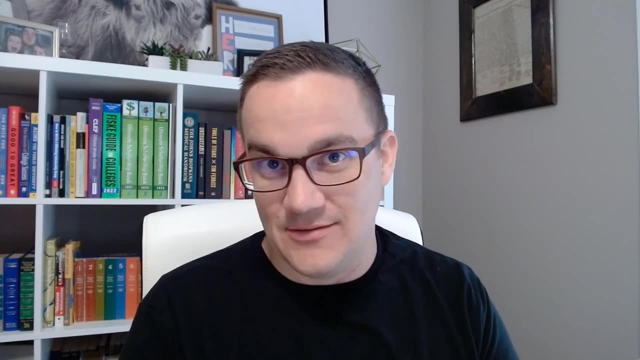 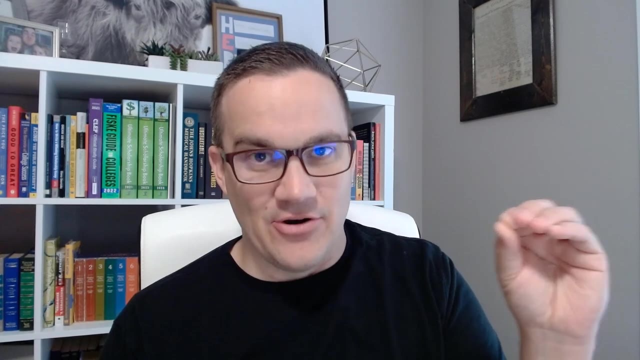 new material, because a lot of it you already know just from life experience. Now, in business, for example, there are classes like business ethics. Well, a business ethics class it's going to say: hey, here's this scenario, You're testing out of a class. Here's this scenario, What is the? 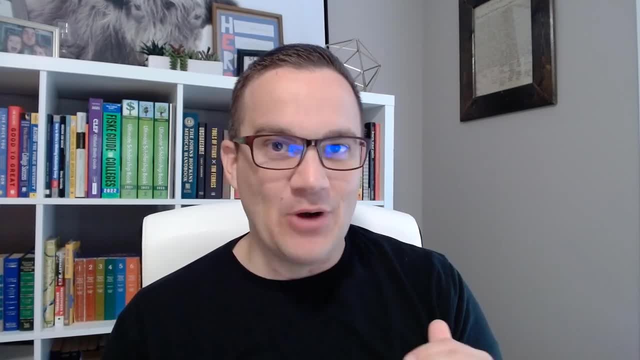 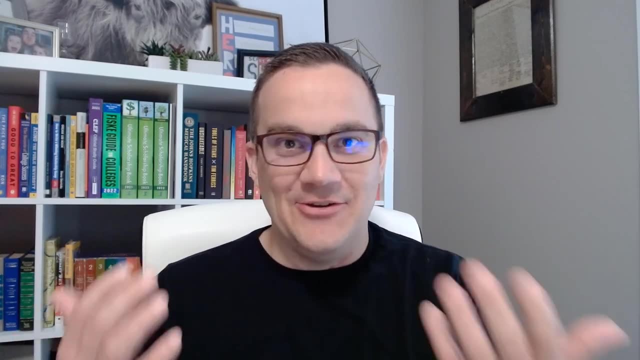 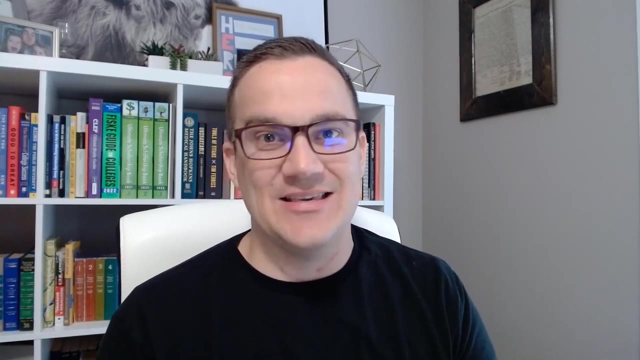 most ethical or honest way to solve this problem- A, B, C or D? Well, if you have common sense and you have any integrity, you're going to know the answer to that question without doing any study. Now there are going to be a few classes. 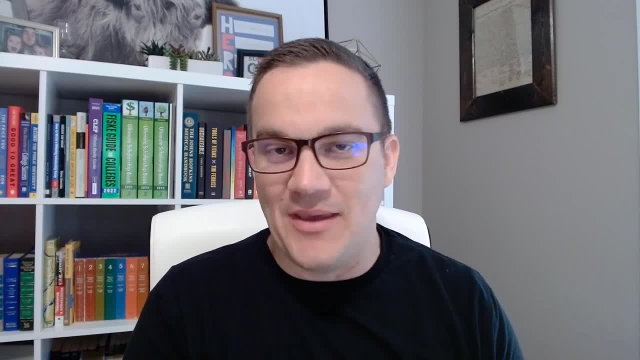 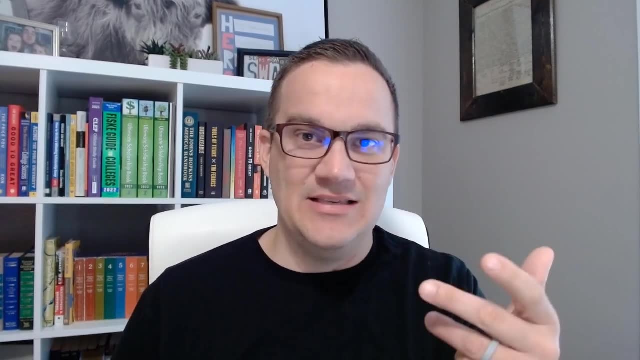 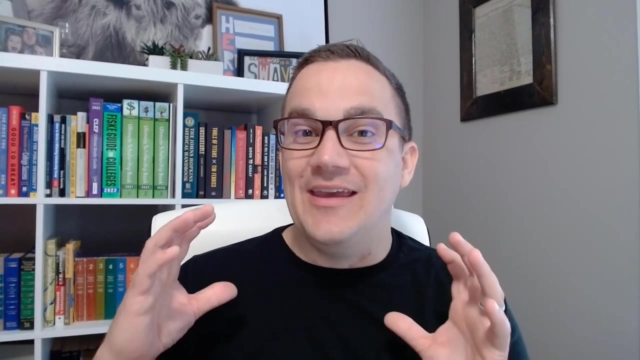 like business law, where you have to learn legal stuff behind business, but those can be learned quickly. Since you're earning less math, less science, less English, less history credits or taking less of those classes, you can generally go really quick. So in a nutshell, in my opinion, 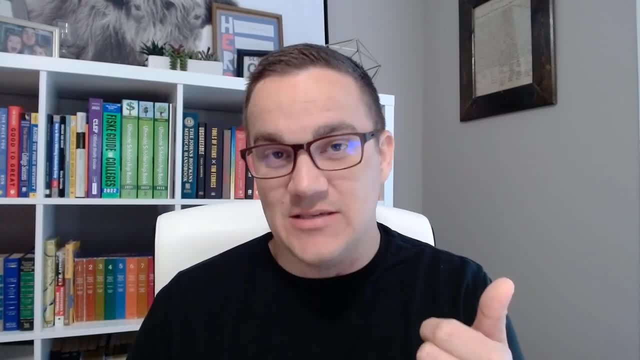 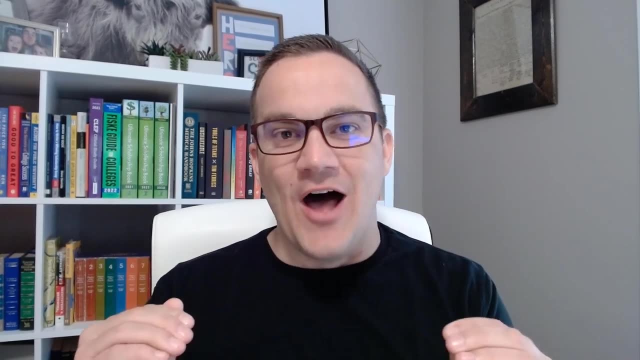 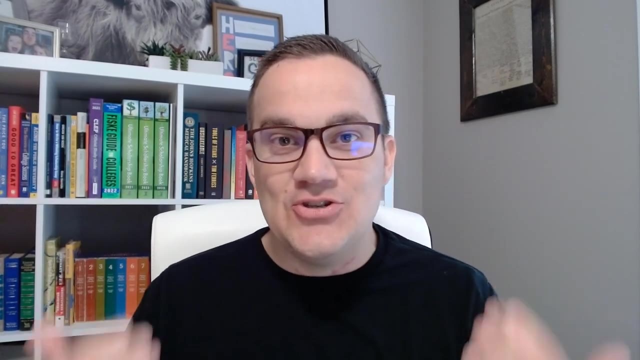 competency-based programs- 100% competency-based- and business degrees. you combine those two together and you can absolutely fly. Now there's a catch to all of this: Schools, even if you choose the right school and you choose the right, major universities don't want you to graduate faster The longer you're in school. 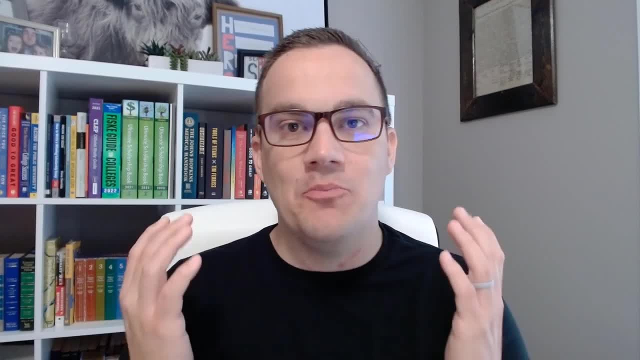 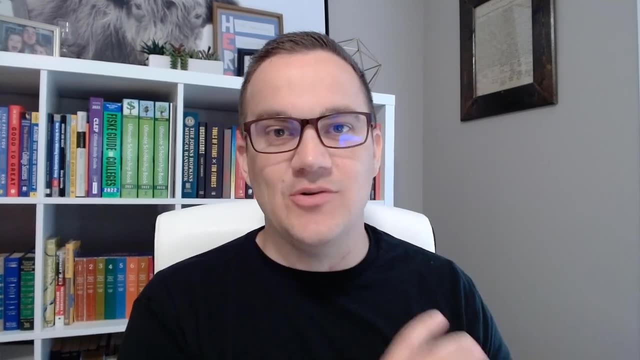 the more money they make and unfortunately, universities are businesses. So here is the deal: If you go, enroll in these programs and try to do it the school's way, read the textbooks, do the homework, the quizzes, follow the study guides and lesson plans and all.